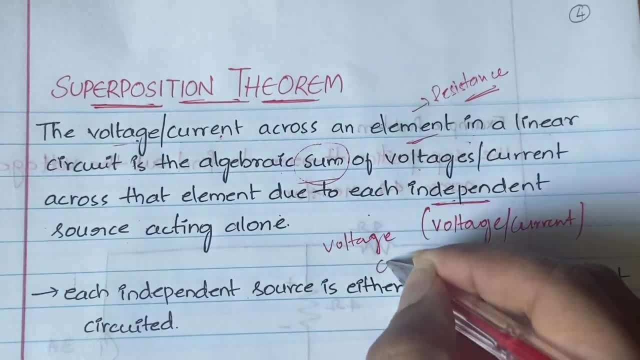 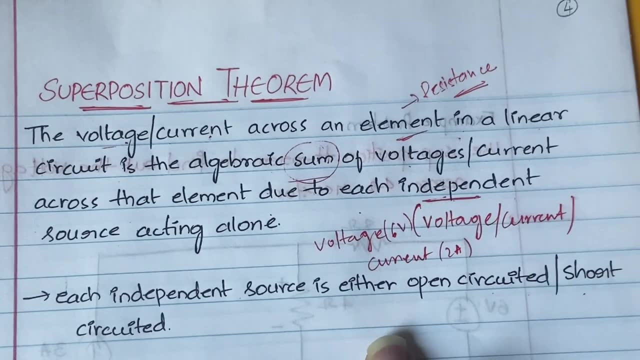 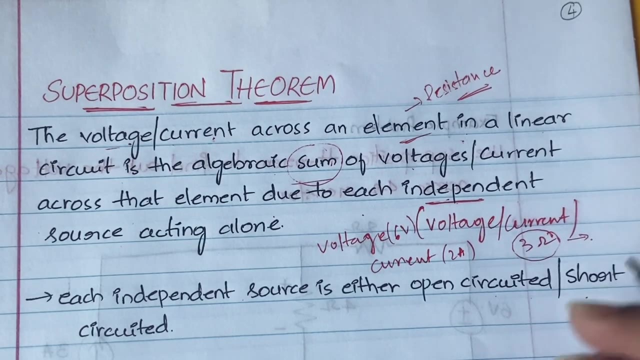 one is voltage and the other independent source is some current, some 2 amperes of current and 6 volts of voltage. let us assume so. and we have a resistor with 3 ohms of resistance. so on this resistor, whatever the voltage or whatever the current is, that will be equal. 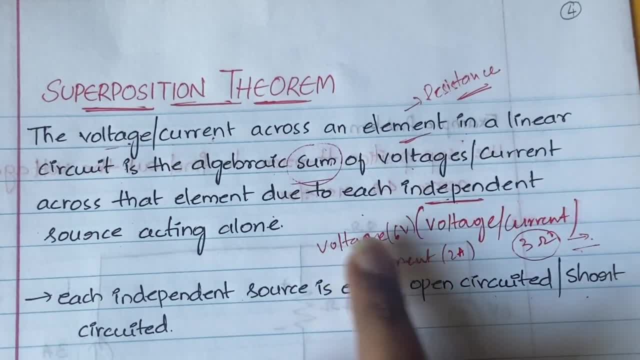 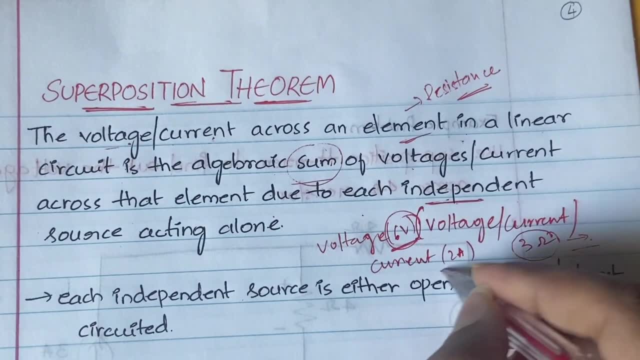 to the sum of algebraic- sorry, the algebraic- sum of voltages when they are acting alone, that is, when 6 volts alone is acting how much, when 2 amperes alone is having how much. when you add both of them, then you will be getting the voltage. 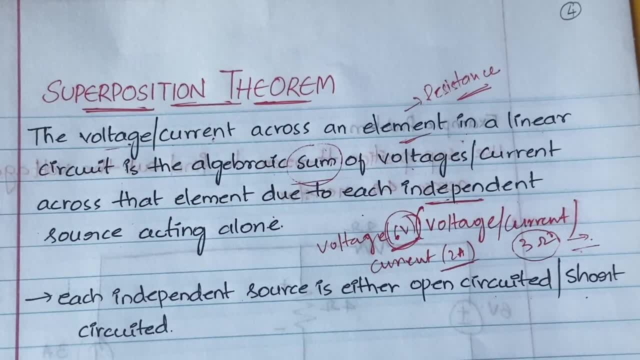 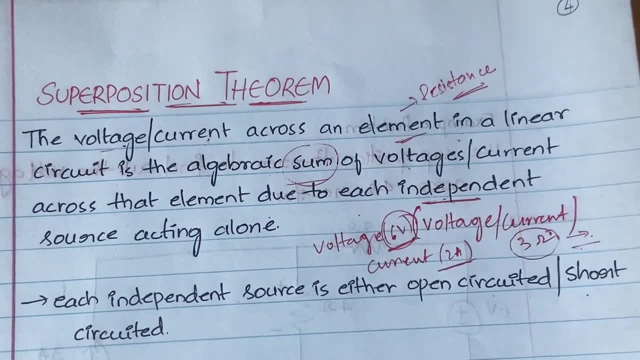 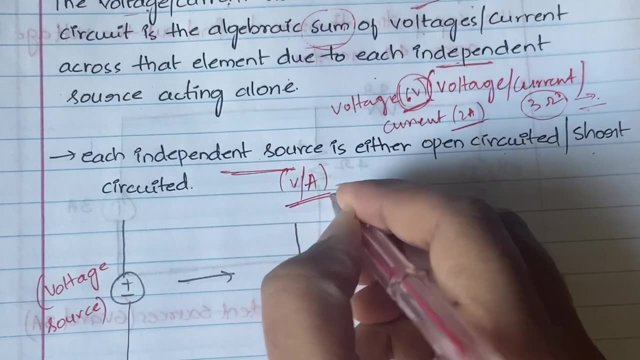 So this is the voltage or current across that 3 ohms resistor. okay, maybe you guys might not still be clear about it. just leave it after example, you will understand it more clearly. So what did I say here? Each independent source. independent source could be either a voltage or a current source. 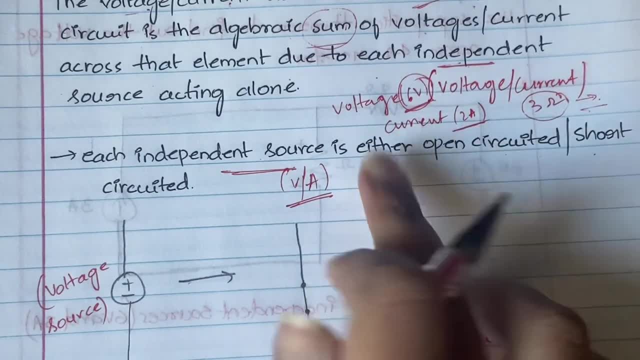 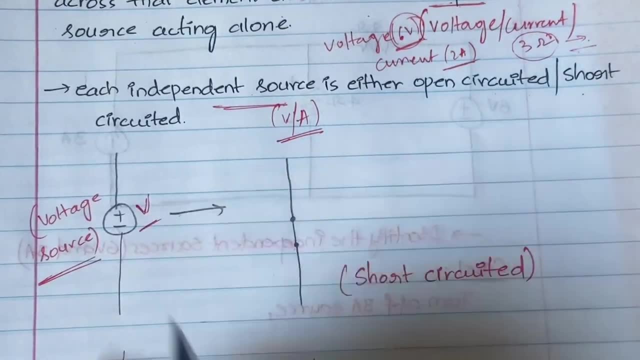 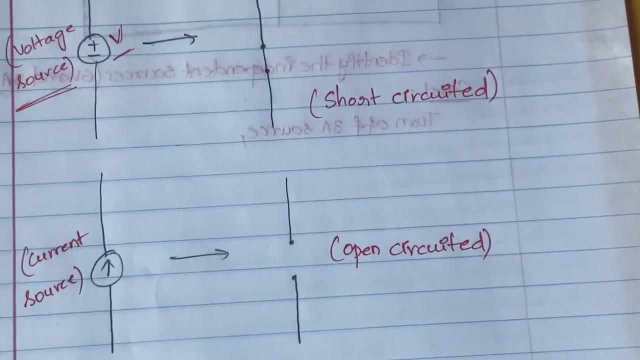 so each independent source will either be open circuited or it will be short circuited. so when do you short circuit and when do you open circuit? suppose if it is a voltage source, okay source, in that case you will short circuit it, okay. and if it is a current source in. 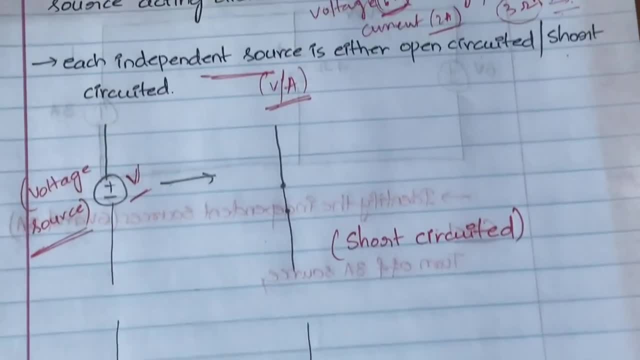 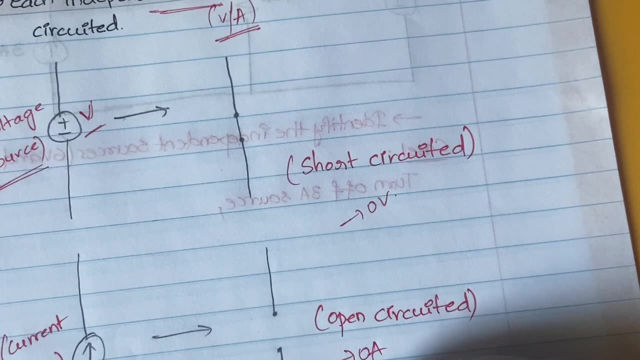 that case you will open circuit it. okay, that means if it is a voltage source, you will be replacing it with 0 volts and if it is a current source, you will be replacing it with 0 amperes. okay, and do not turn off the dependent sources. do not touch the dependent. 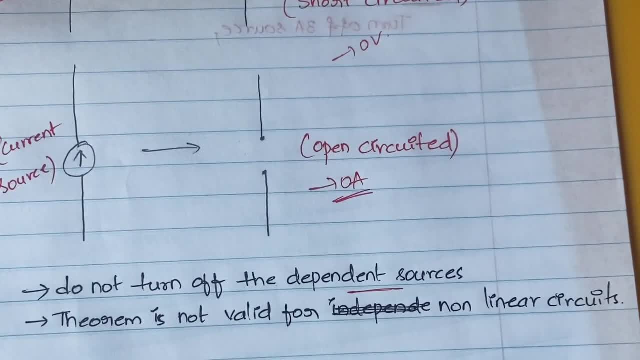 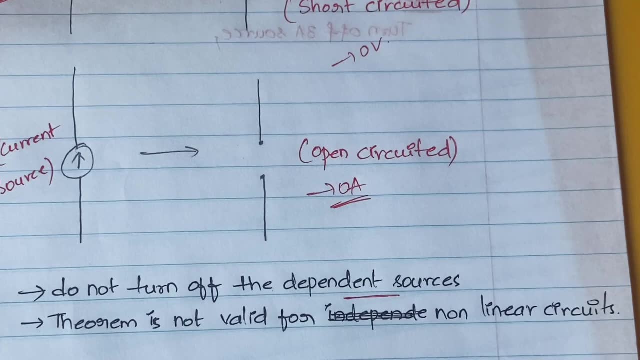 sources. just leave them as they are, and this theorem is not valid if the circuit is a non-linear circuit. it is valid only for linear circuits. okay, now let us try to understand this with an example. this is our example problem. use superposition theorem to find. 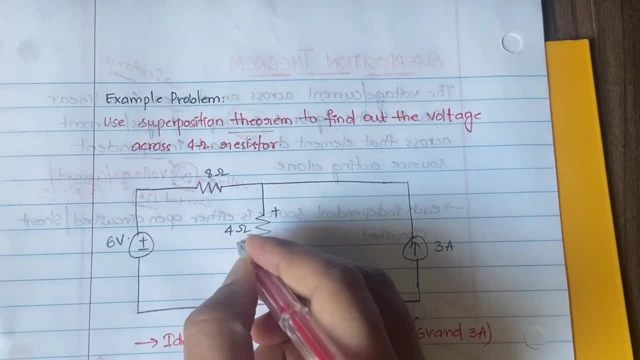 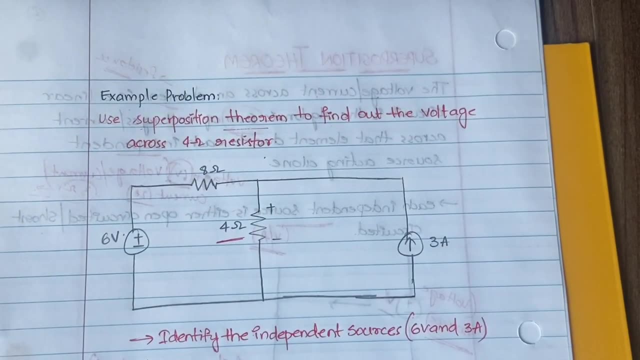 out the voltage across 4 ohms resistor. where is 4 ohms resistor? here it is. so the voltage across this 4 ohms resistor. we have to find how By using the superposition theorem. so first, what you need to do is you need to find out the voltage across this 4 ohms resistor. 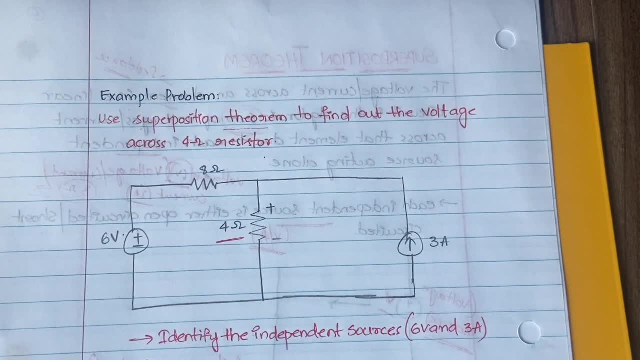 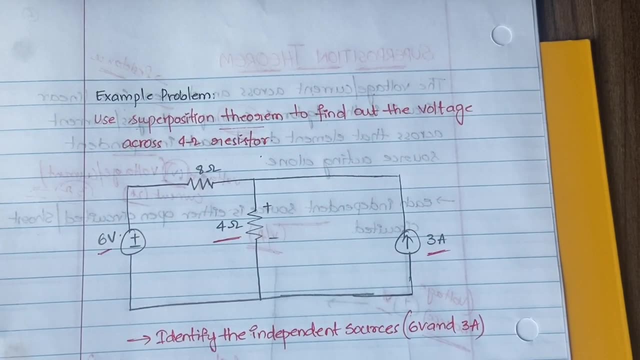 you have to do: identify the independent sources. what are the independent sources in the circuit? 6 volts is one independent source and 3 ohms is one independent source. okay, so now what we have to do? we have to turn off each independent source and find. 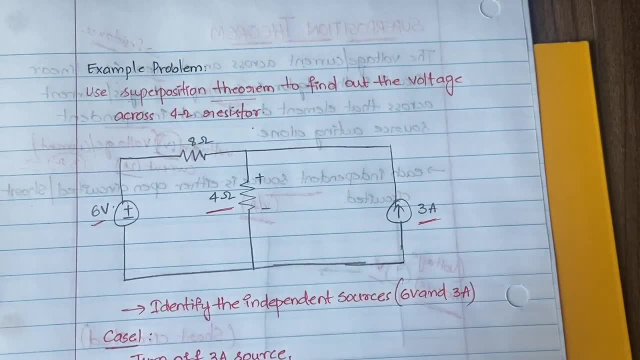 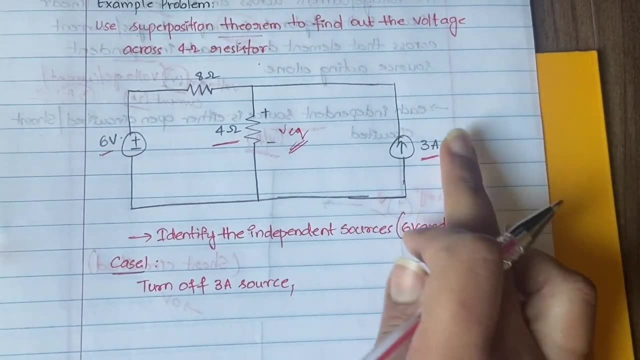 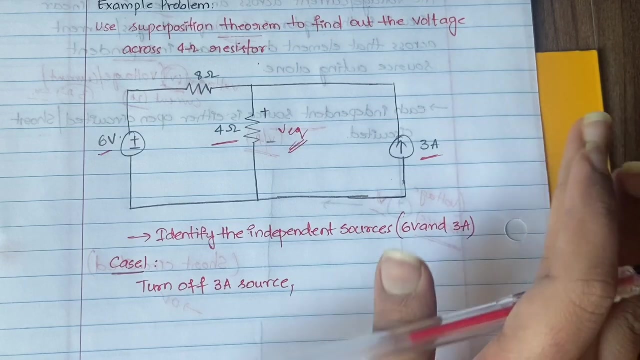 out the voltage in each case and then add the voltages in both the cases so that you will get the total voltage right. so let us see. first let us consider turning off this 3 ohms diagram. I mean, sorry, 3 ohms current source. okay, we are turning off the 3 ohms. 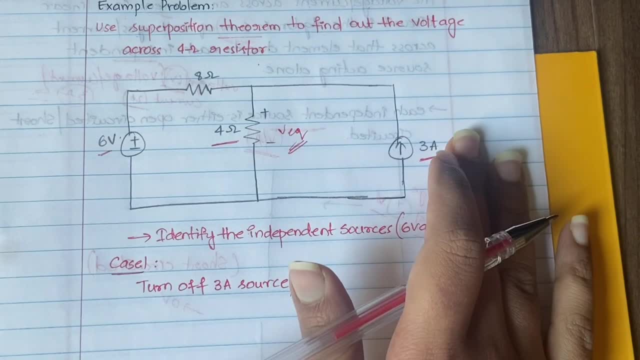 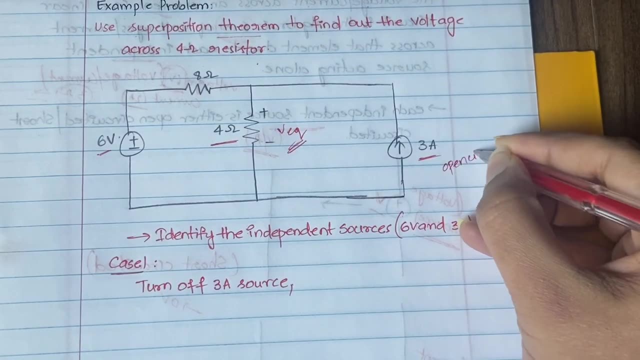 current source. so when we are like, what do we say, when we are turning off the current source, what we will do? We will do the open circuit right. so if it is a voltage source, we will do, for voltage source we will do short circuit. but for current source, what? 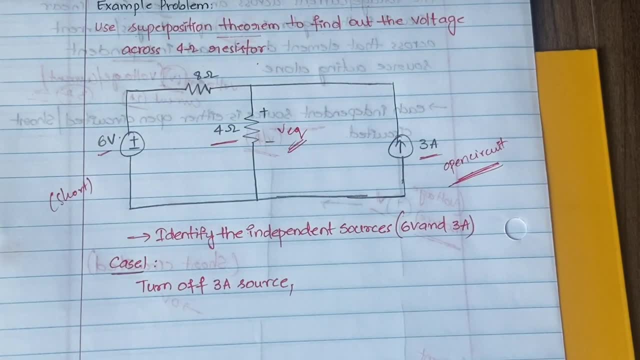 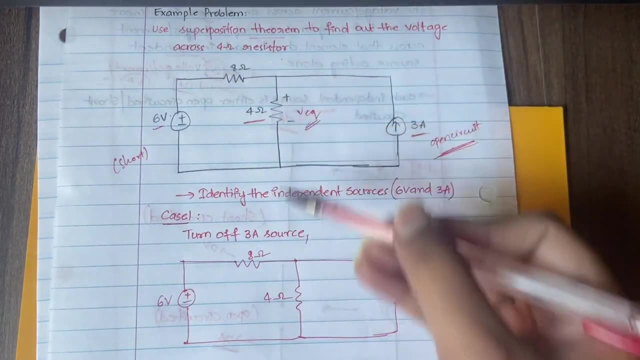 we are doing? We are doing open circuit. so now the new circuit diagram will be. now the new circuit diagram will be like this: We removed this 3 ampere source and we did it as a open circuit. Other 8 amps, 4 amps, 6 volts. everything will be as it is. 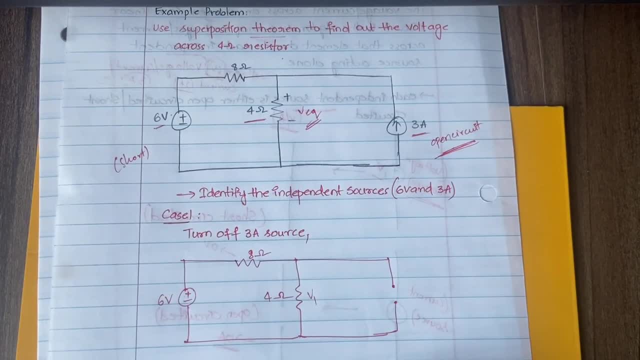 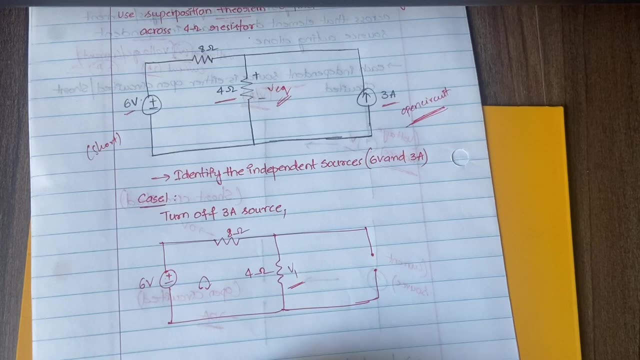 We just removed this And let us consider the voltage as V1 over here. Now our task is to find out V1.. Okay, Now how do you find out V1?? For example, assume the current passing over here is I1.. 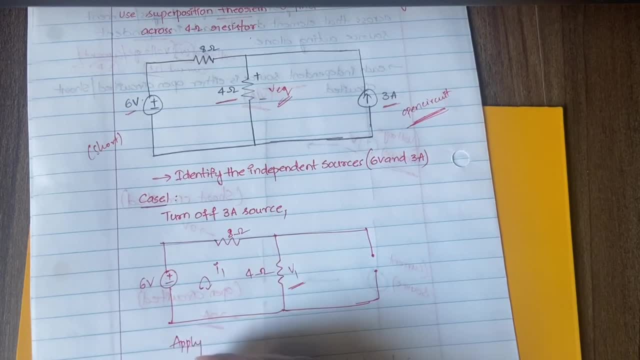 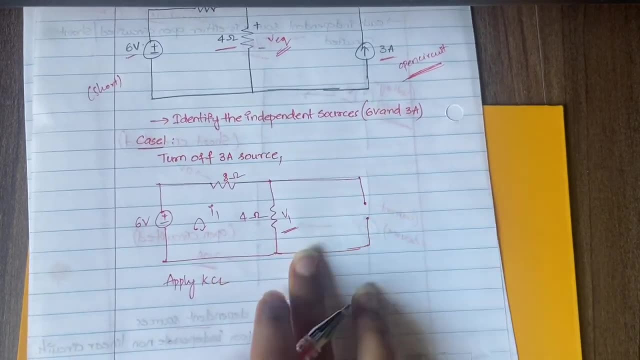 Okay, And now apply KCL. Apply KCL in this circuit. Now, for time being, forget about this circuit. Just consider this circuit and apply KCL in this circuit. However, here it is open circuit, So the current will be 0 in this loop. 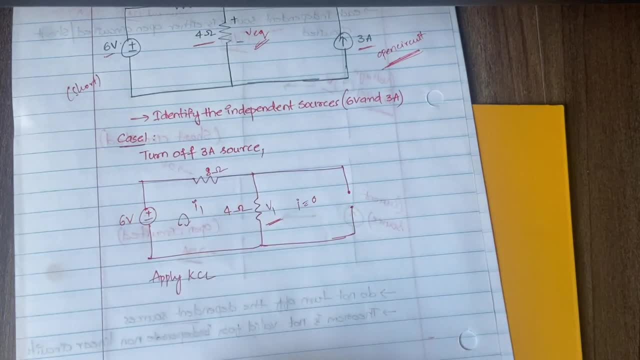 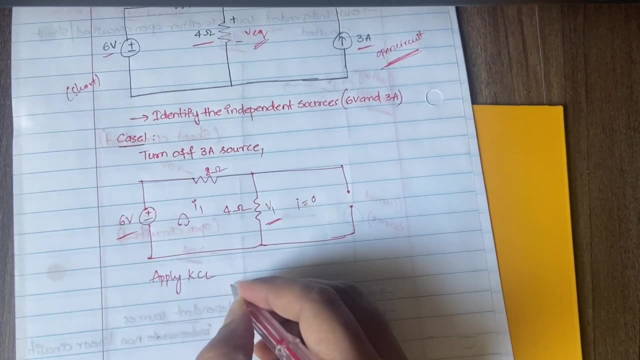 Okay, That means you are applying KCL only in this loop, Right? So how do you write the KCL equation? So 6 volts, I am sorry, Sorry for confusing you guys. Apply KVL. KVL means voltage. 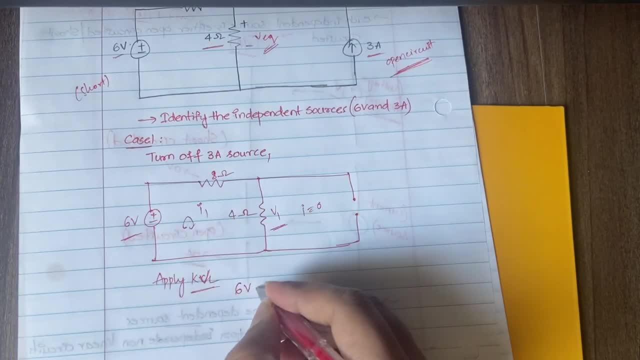 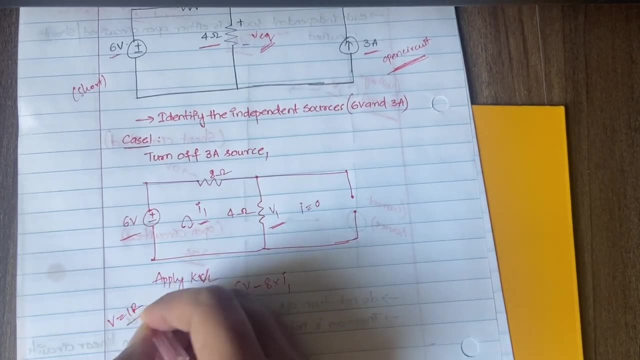 Right, So what you will do? 6 volts minus 8.. Times, What is the current here? I1. V is equal to IR formula. I1 into resistance is 8 ohms Minus. Okay, 4 into. 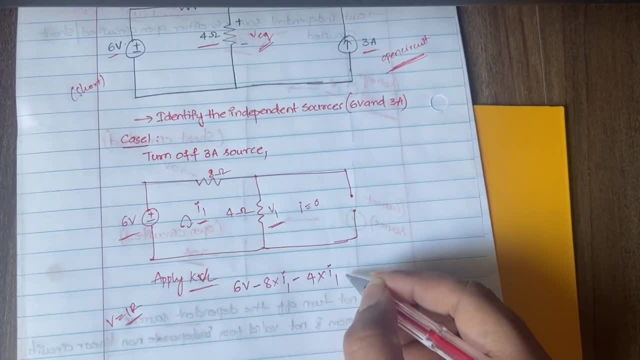 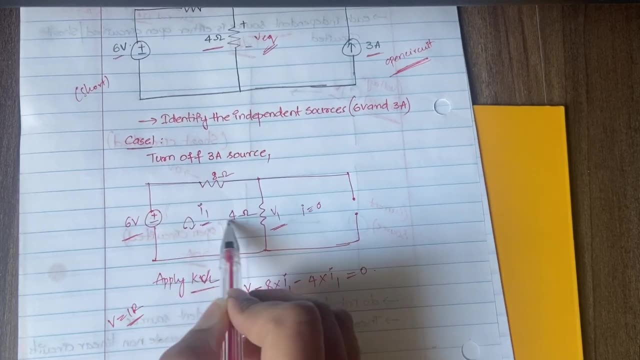 What is I1? here again, What is the current? here again, I1. Is equal to 0. Okay, Why we got minus Sine convention. You know right, Current always flows from higher potential to lower potential, So the potential will be dropping. 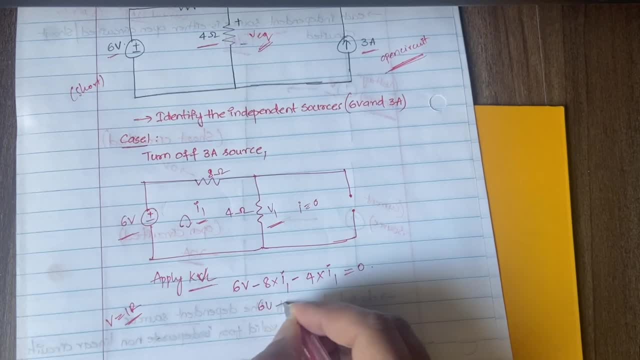 So, as a result, you are taking it as minus like this: So 6 volts minus 8 I1.. Minus 4 I1. You will get 12 I1 is equal to 0.. Okay, Take it as 6 only. 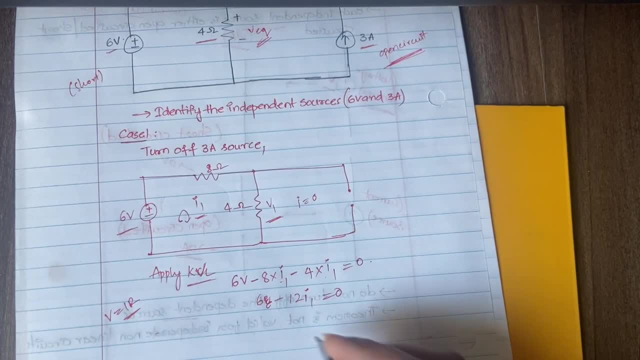 Again, if you see V you will get confused. that V is again another variable. So you will get: 6 is equal to 12, I. From this you will get: I is equal to 0.5 amperes. Right. 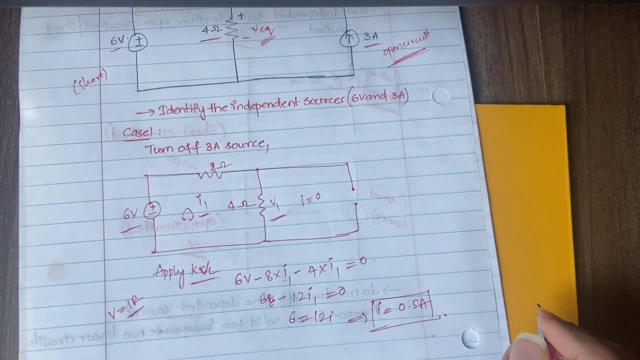 When you send 12 to this, it's better 1 by 2, which is 0.5 amperes. But what is your task here? Your task is to find out V1.. Right, So how do you find V? 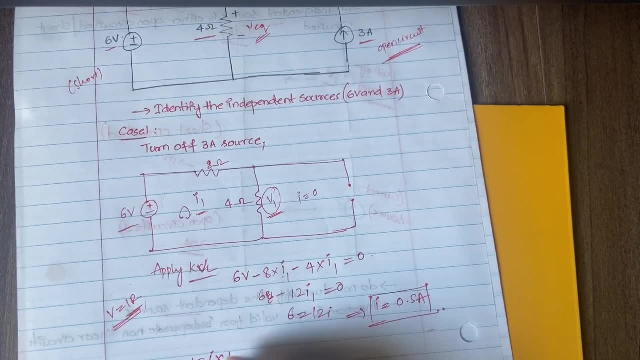 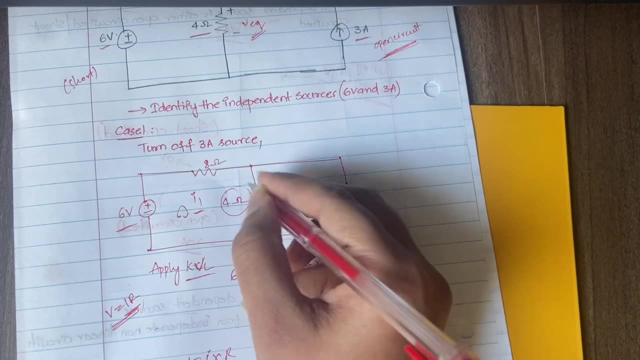 V is equal to I into R. V is equal to I into R. What is the I? you got 0.5.. And what is the resistance? What is the resistance over here? at this point, Don't forget about this V1, right. 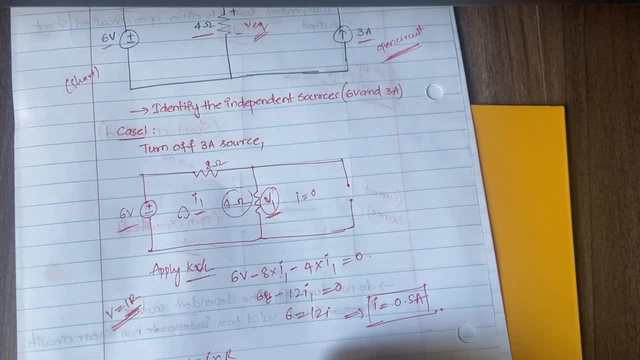 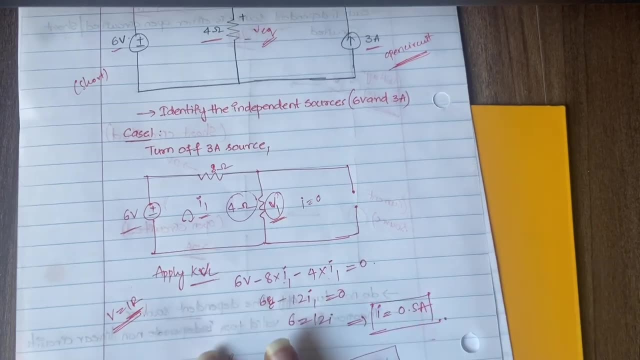 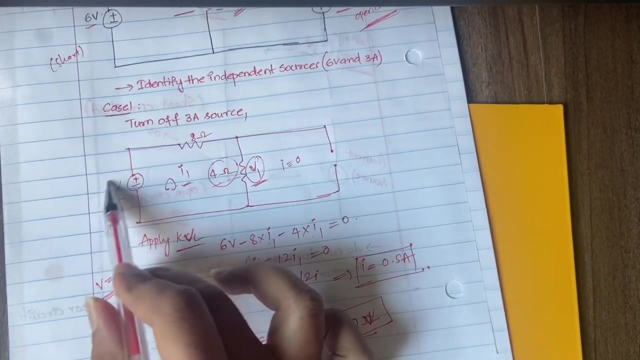 At 4 ohms resistor, you are finding out. So 0.5 into 4, which is equal to 2 volts. So V1 is equal to how much 2 volts? Okay, So the voltage acting on 4 ohms resistor due to the 6 volts independent sources, how much? 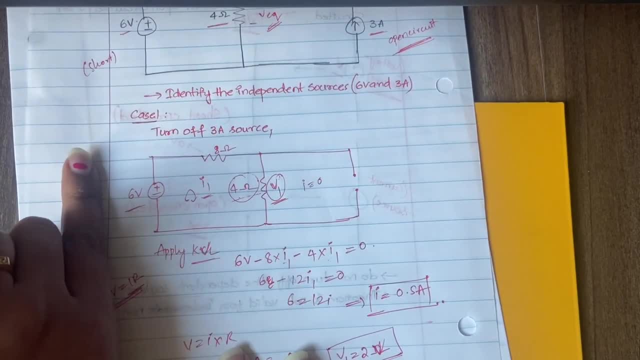 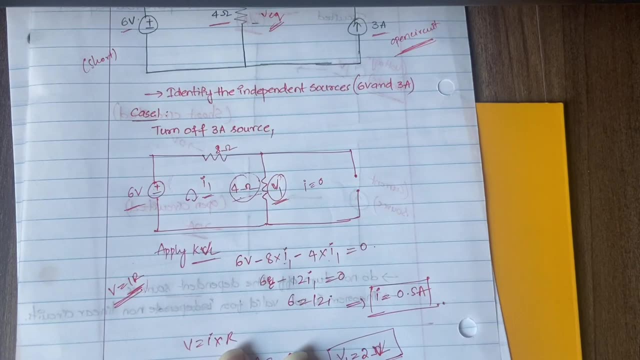 2 volts, 2 volts. In the same way, you have to Start circuit this and you have to consider this 3 ohms current source and find out V2, and then you will have to add V1 and V2.. Okay, 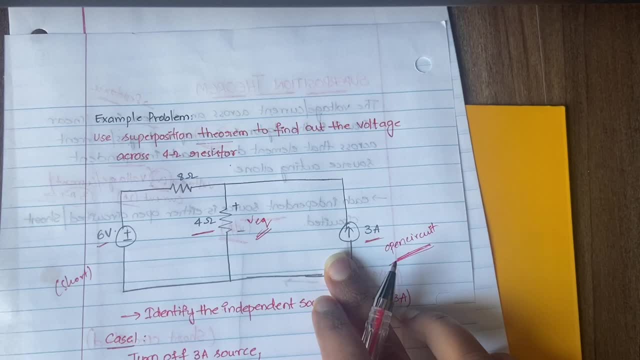 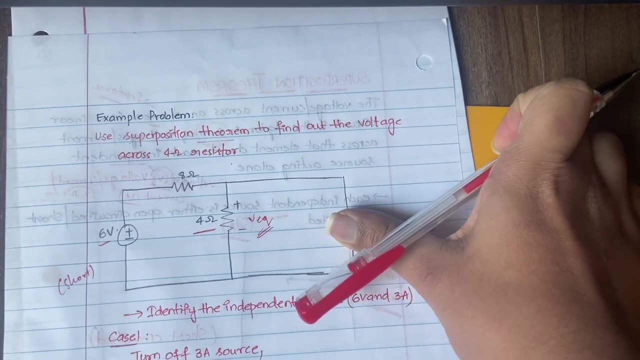 Very simple guys. This is the original diagram. So in this we have how many independent sources? 2 independent sources. So you will be getting 2 cases. First case: we turned off the current source and in the second case we will turn off the voltage source. 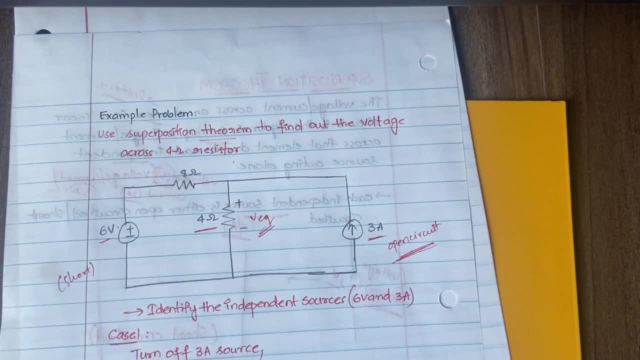 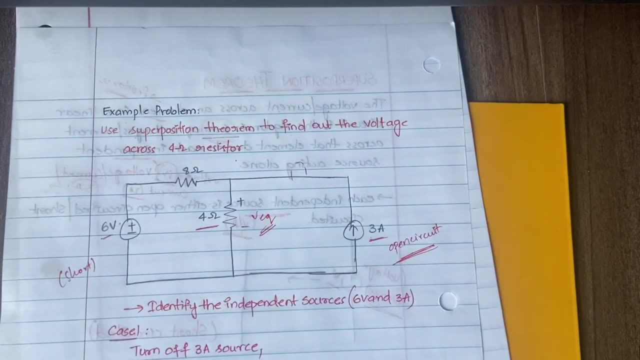 Suppose, if this circuit diagram is having 3 independent sources, Suppose here it is having 1 more current source, Then you will have to do 3 cases: First, turn this off, second, this, third, this, Okay, Sorry, How many independent sources are there? 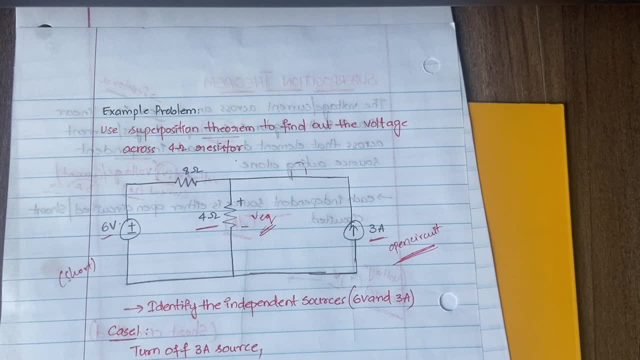 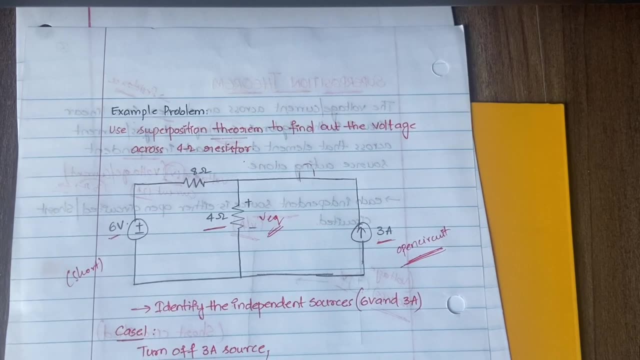 You have to turn off all those independent sources and you have to find out the voltage in each case and add all the voltages. Very simple Now, in our second case, what we have to do: We have to keep this one and we have to short circuit this voltage source. 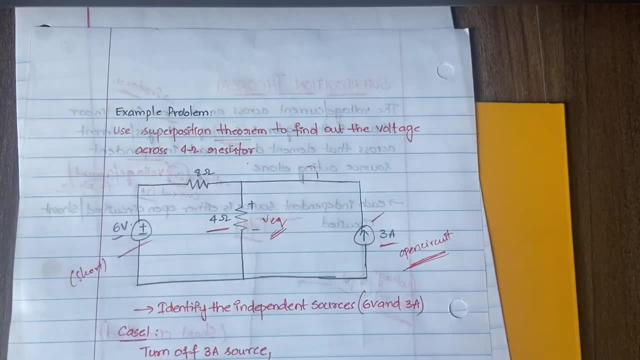 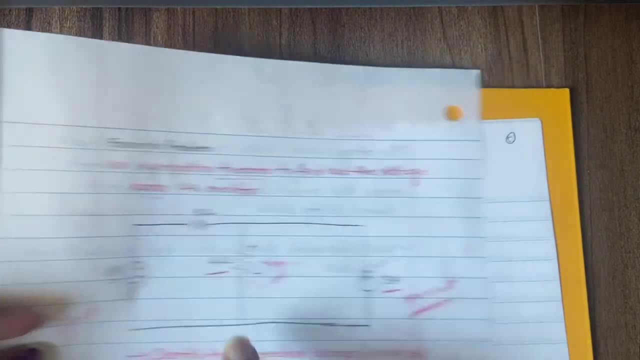 Right, So if we short circuit this voltage source, let us see what is our new diagram. This is the diagram that we got After short, after short circuiting this voltage source. see, this is our original diagram and from this original diagram we got this one. 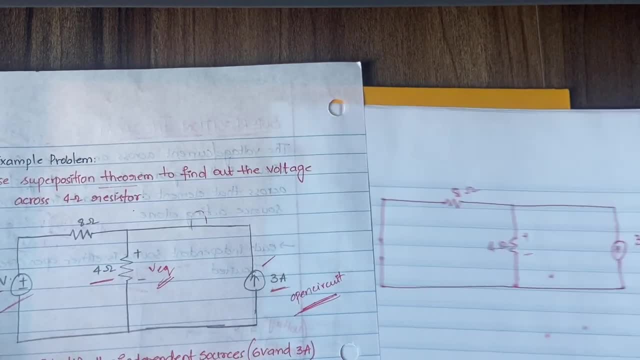 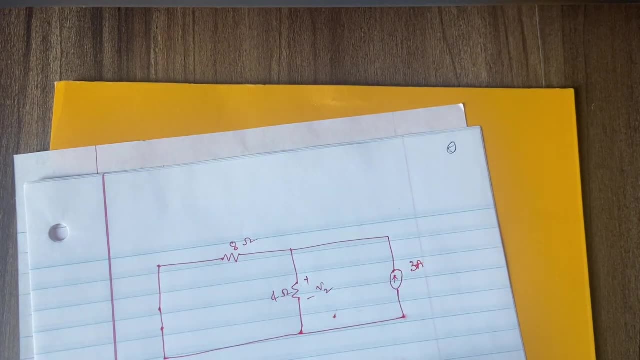 Okay, That means we just removed the source, The other, everything is as it is Now. let us see. Now let us consider the voltage as V2 over here And now let's find, let's calculate the voltage. Okay. 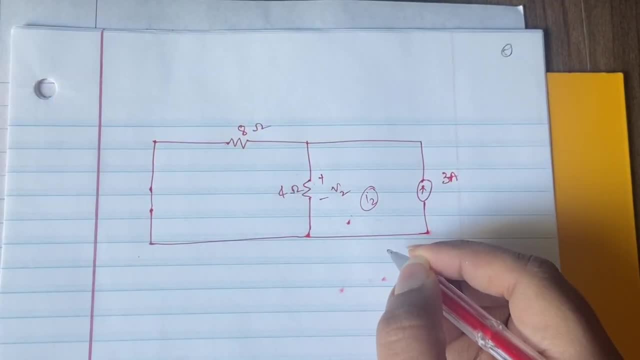 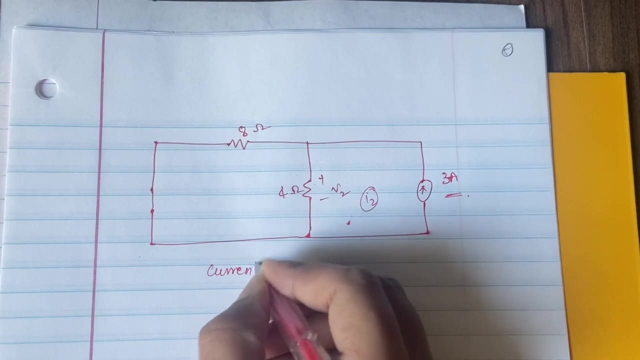 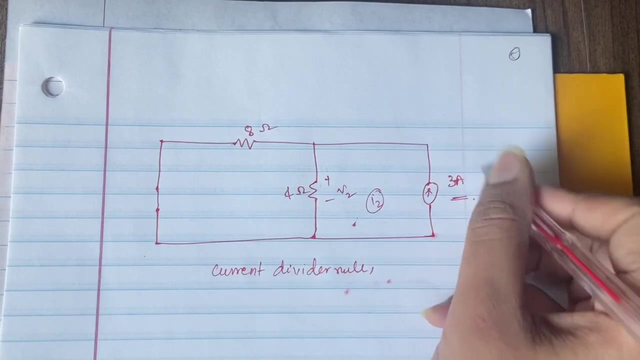 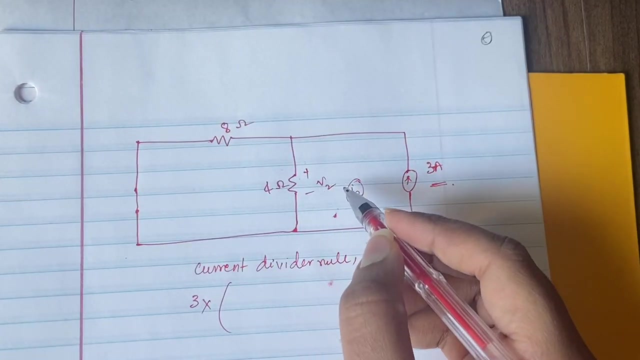 Consider current as I2.. Okay, And we already have one current over here. Right, So let us apply Current divider rule. If you apply current divider rule, so what is the original current? what is the entering current 3 amperes into? what is the resistance? you have here? 8 ohms, right, 8 divided by 8 plus 4.. 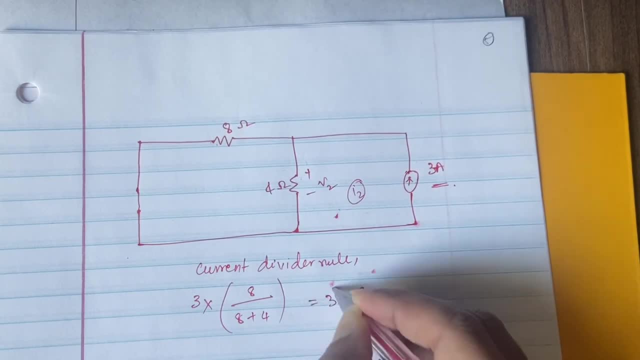 Okay, That means you will get 3 into 8 by 12. So you will be getting 2 amperes. So you will be getting 2 amps as the I2.. So I2 is equal to how much? 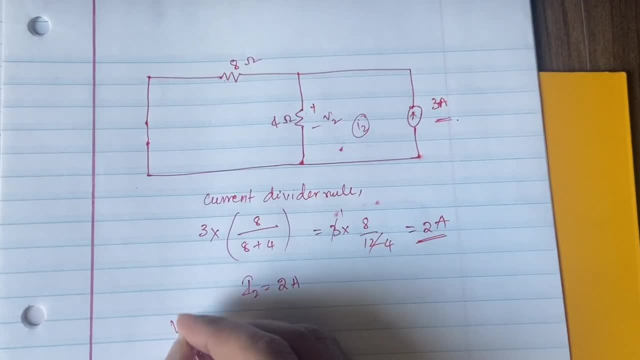 2 amps. But your task is not to just find out I2.. Your task is to find out V2.. V2 is equal to I2 times R. R is nothing but here. what 4 ohms? Because V2 is here, right. 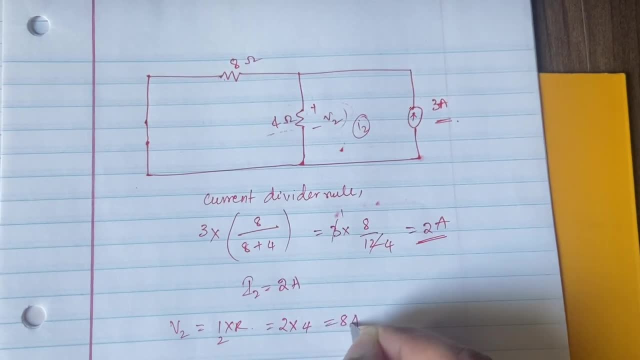 So it means 2 into 4.. That means how much You will get it as 8 volts. Okay, So V2 is equal to 8 volts. And previously, what did we get for V1?? We got V1.. 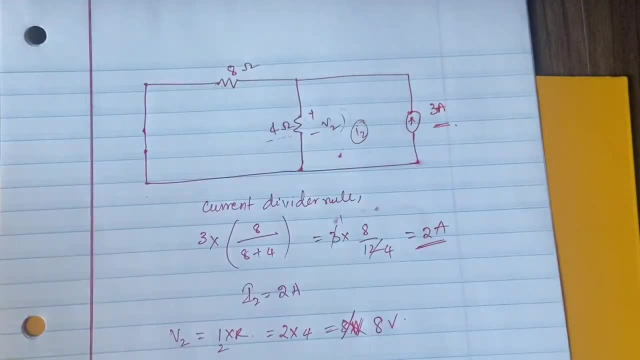 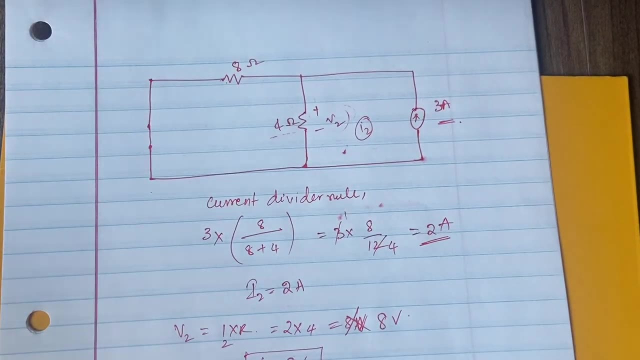 V2. V2. V1 as 2 volts. How? By removing these 3 amps, Okay Now by removing this 6 volt source, we are getting V2 as 8.. So what does superposition theorem says? 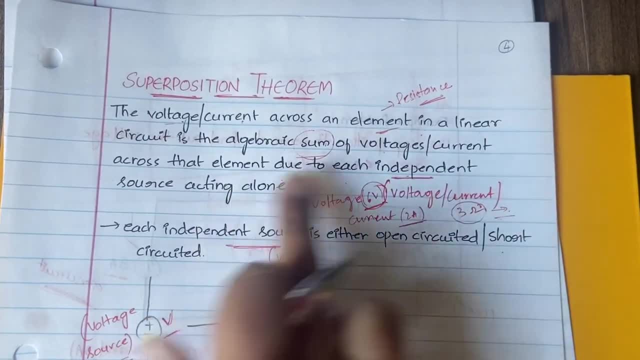 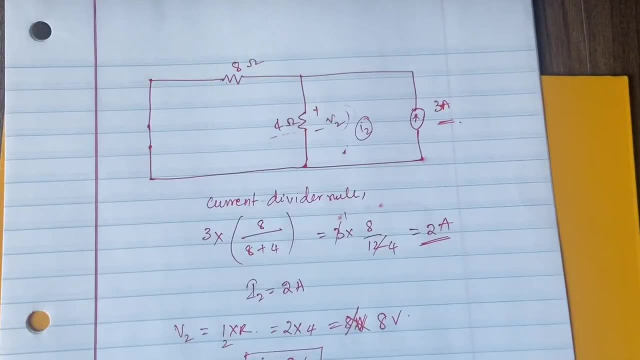 Algebraic sum of voltages acting due to each whatever voltages or current acting due to each independent source alone. Each independent source alone, right? So that means total voltage will be equal to V1 plus V2, which is equal to 2 plus 8,. 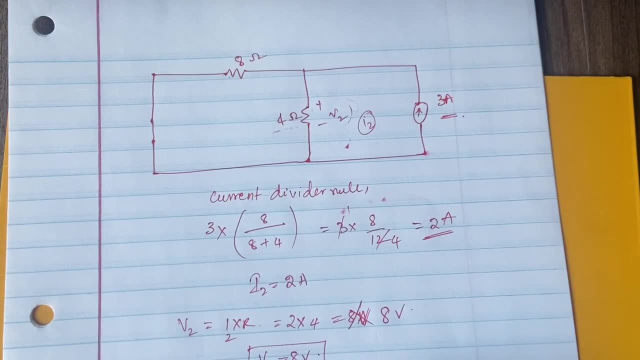 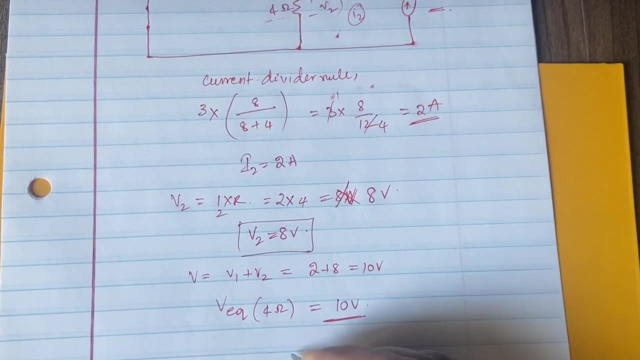 which is equal to 10 volts. So V equivalent or voltage at 4 ohms resistor is equal to how much 10 volts by superposition theorem? Okay, Now I hope you guys are clear about the definition of superposition theorem.